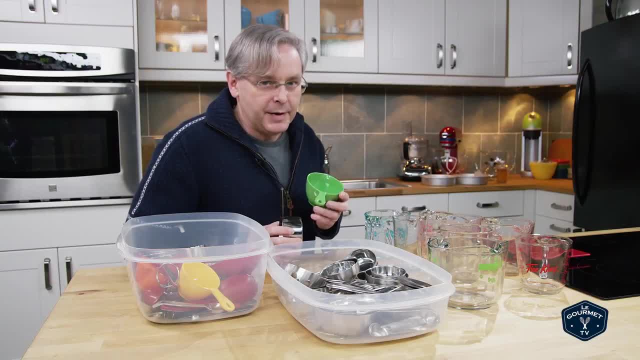 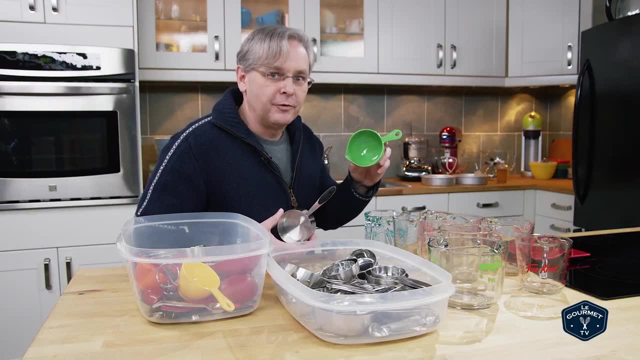 In most cases the measuring difference doesn't really matter, especially if you're only doing one or two cups of flour or sugar. The difference between 240 milliliters and 250 milliliters is two teaspoons, So not a whole lot. 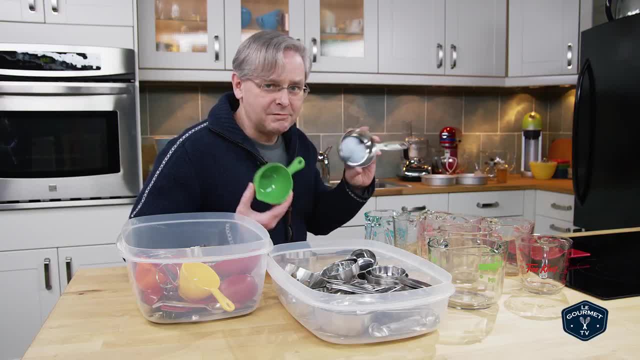 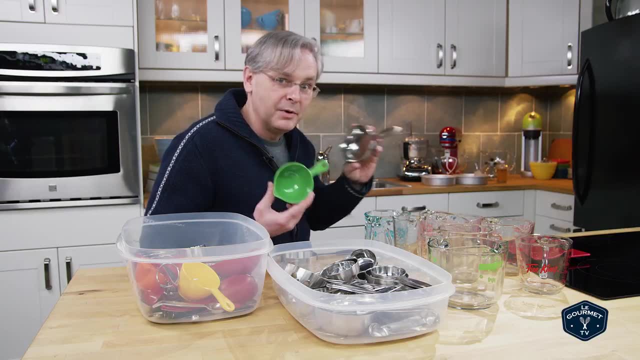 But I find it very interesting that even within the United States they've got two different, competing cups And if you went into your kitchen cupboard right now and took a look, you might have cups in both sizes, And if you're in Canada you will have cups in all three sizes. 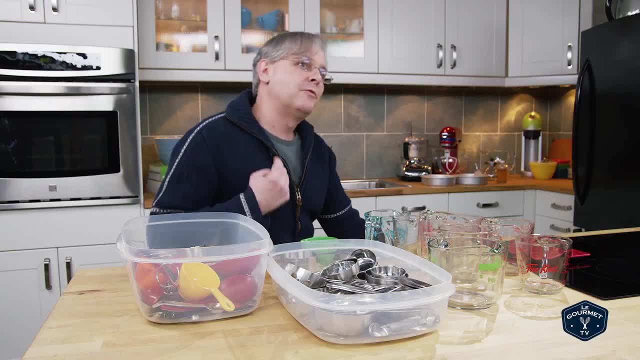 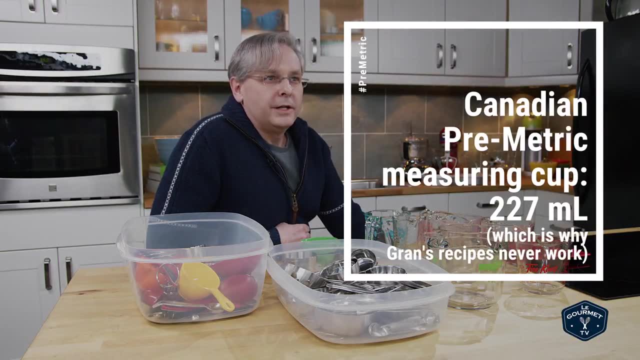 If you're in Canada you may even have four sizes of measuring cups, because before Canada went metric in the 90s, In the 1970s our measuring cup was 227 milliliters or 230 milliliters, so even smaller. 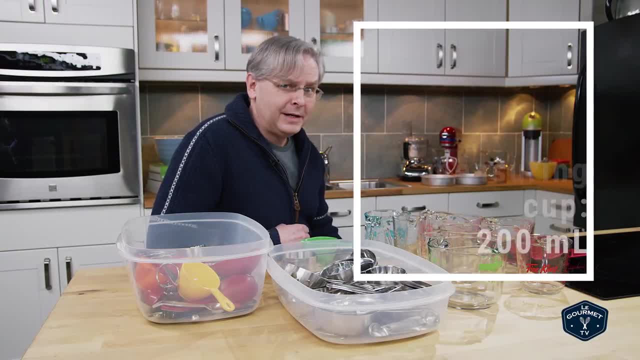 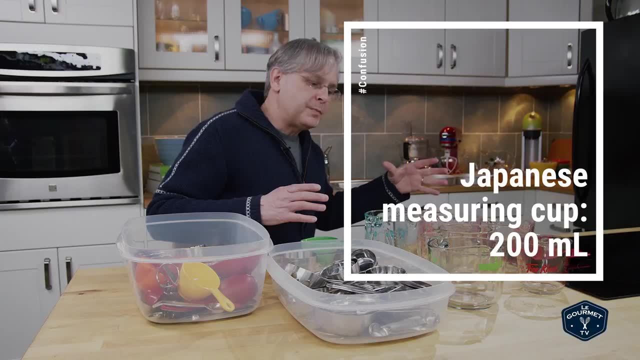 I'll put that up on the screen in case I got it wrong. If you're in Japan, they've got an even smaller measuring cup, So we stopped using cups. We still put cups in, but we put the metric equivalent beside it. 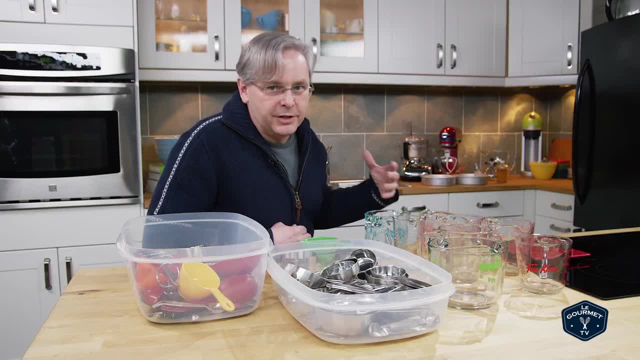 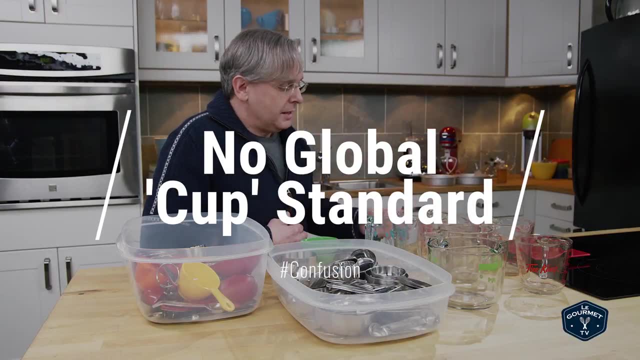 So everyone who's yelling at me and saying a measuring cup, a one cup measure, is not 250 milliliters. The measuring cup that we're using is 250 milliliters. And everyone who's saying they don't know what metric is, that's fine, but it's really. 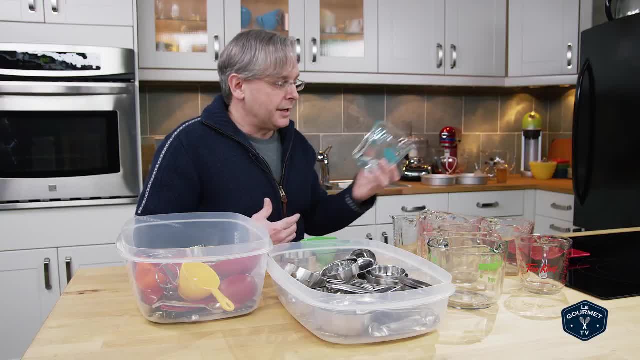 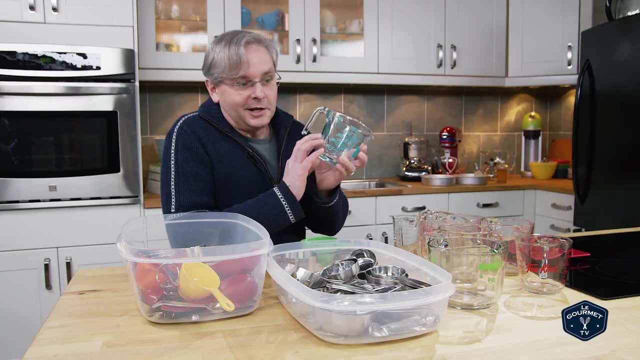 not that difficult, especially since this is a measuring cup that I got in the United States. These are all measuring cups that I got in the United States And on one side is cups and the other side is milliliters. So just turn it around and put 250 milliliters in. 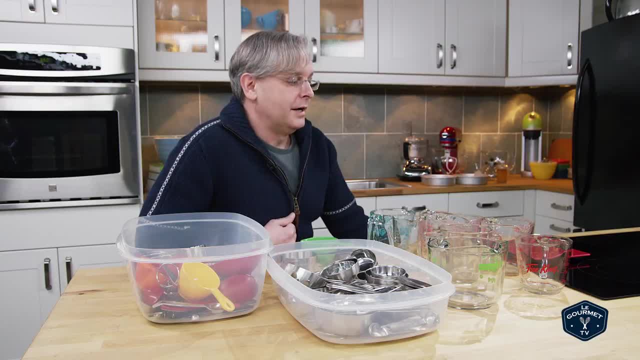 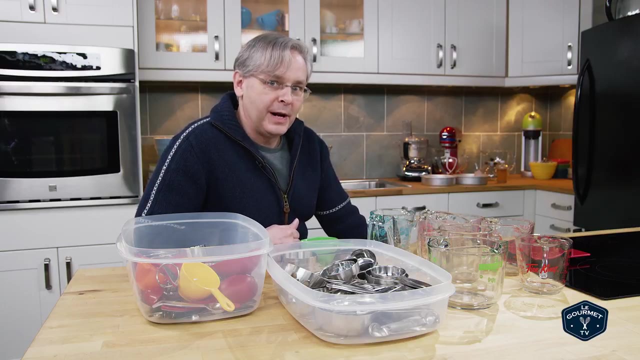 It's really not that difficult to do. I know that's where I'm getting a little bit ranty, but it can get confusing. It's not wrong, It's just different, And we always are now putting the metric so that you can compare and make sure that you've. 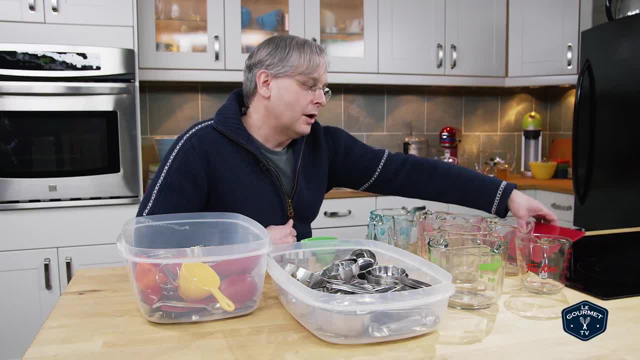 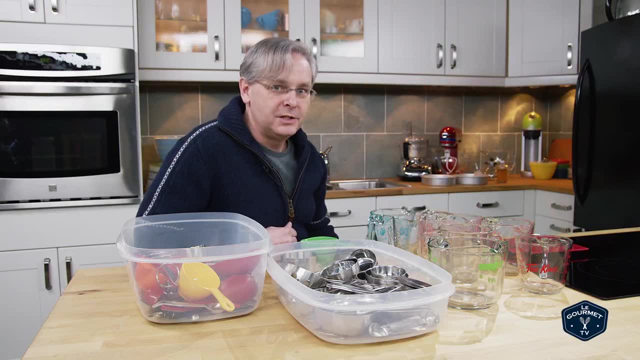 got the right measurements And, as we move forward, more and more of our dry ingredients will be weighed. A quirk of the Canadian change to metric is that we don't weigh dry ingredients like the rest of the world does. We do volume measurements, like the Americans do. 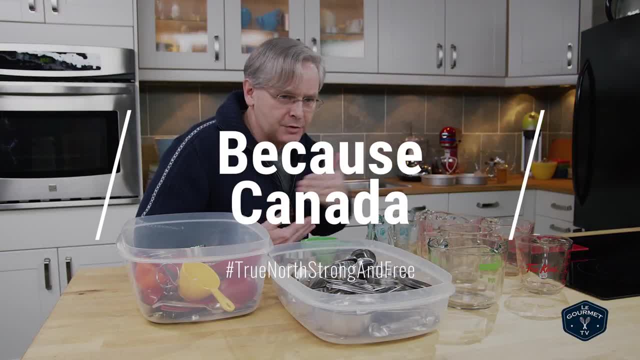 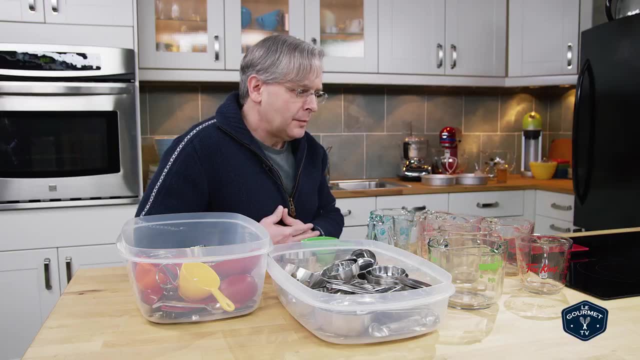 We live in this sort of weird kind of space where you know we pick and choose from a whole bunch of different places. So that's the difference in the one cup measure. I would tell you that if you find a recipe from Australia or New Zealand on the internet, 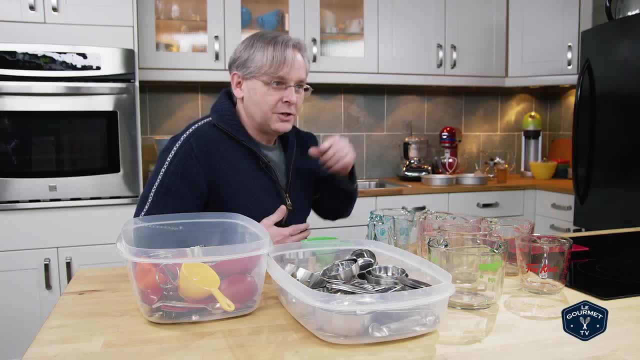 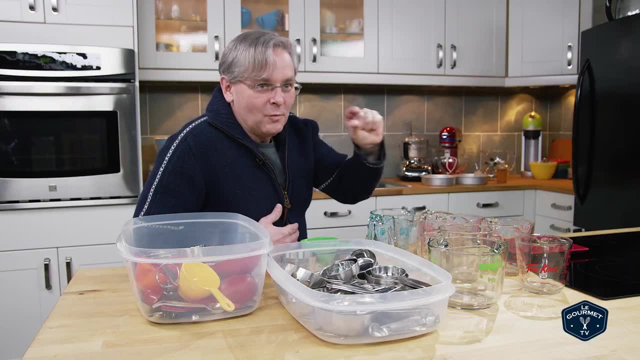 their quarter cup and third cup measurements are different. They chose a different spot from Canada and the United States. So Break out what is a third and a quarter cup. You'd think it would be very easy, but you know, you round up and you round down and 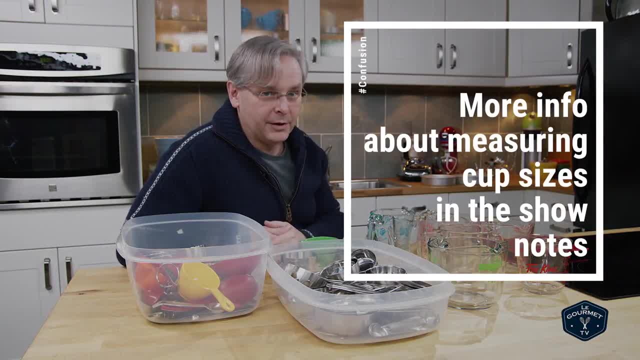 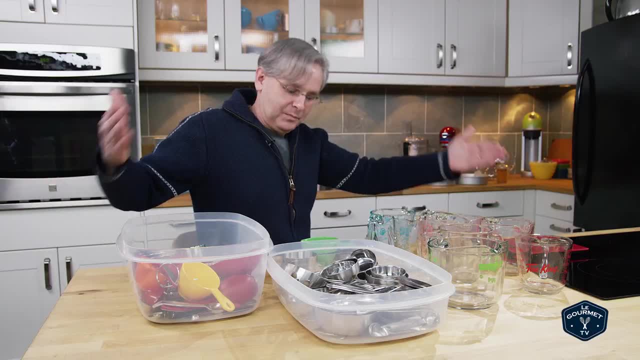 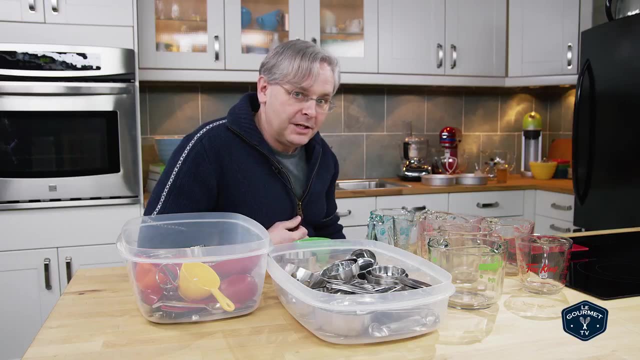 they chose a different spot than we did, which is different than the Americans did. So where am I going with this? All kinds of measuring cups. Take a look and find out what size your measuring cup actually is and then measure accordingly. Take a look at your recipe. 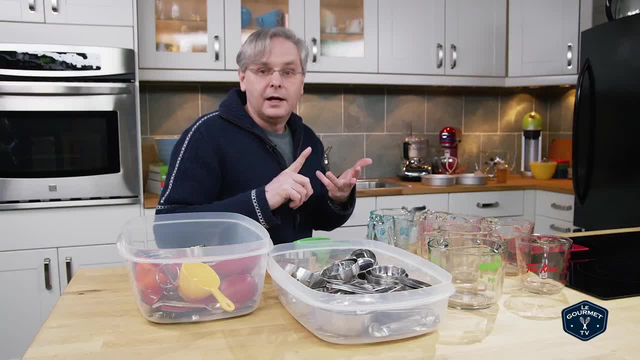 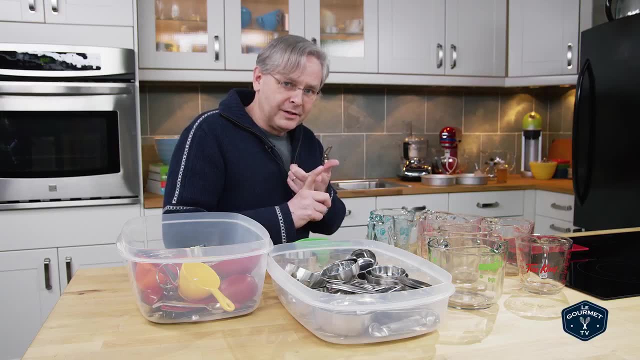 Look at your recipe. Is it from Canada? Is it from Australia? Is it from New Zealand? Um, They also use a different size tablespoon than we do. Is it from England? If it's European, it will be totally metric and you'll have to get a scale which is very 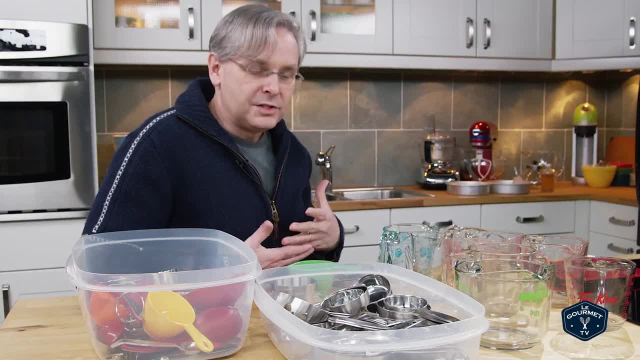 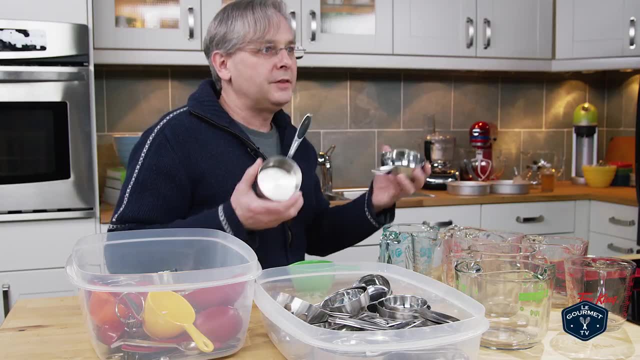 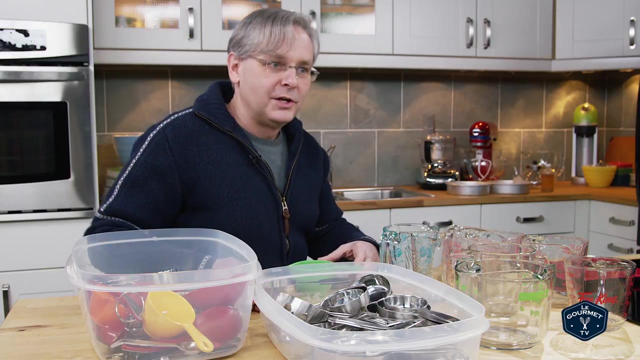 easy to do And a lot of these differences. if you know, if you took this cup- Canadian cup- and this American cup, you filled them with flour, or you handed these to 10 different people and had them fill them with flour and then weighed the results. 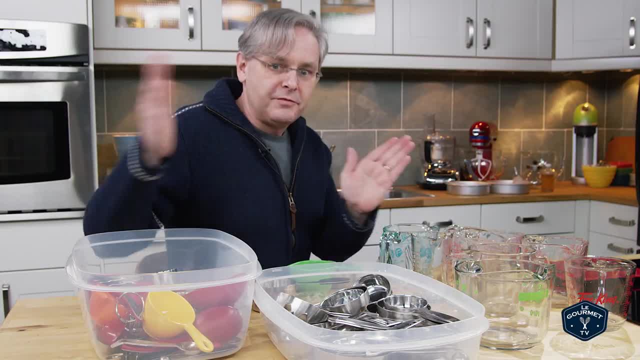 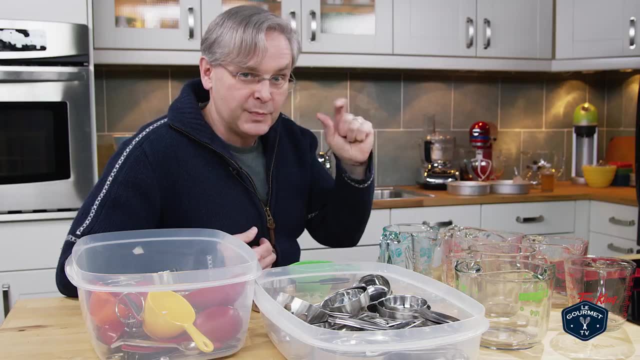 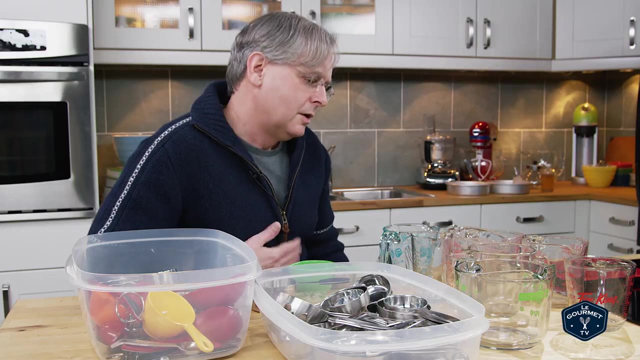 It would be all over the map And you would have this margin of error that was quite wide. A scale decreases that margin of error, makes sure that your recipe is repeatable, especially for baking. For cooking- who measures anything For cooking? you just sort of pour it in and you say, oops, I maybe poured too much in. 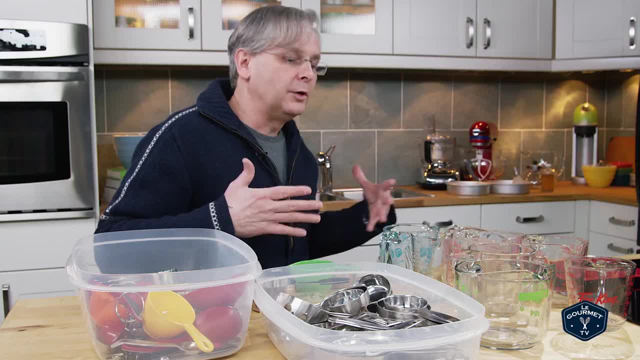 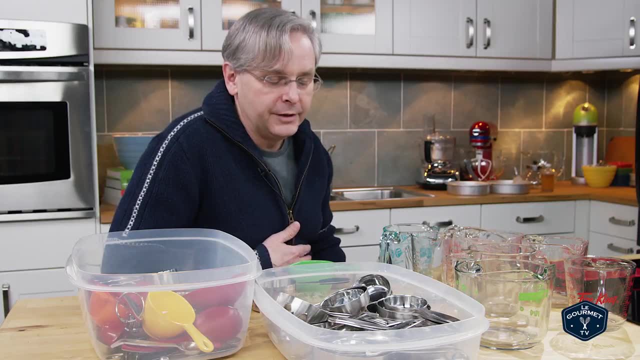 or, you know, maybe I need a splash more. But for baking it is a little bit more important, And for some recipes it's vitally important that you get the right amount of dry ingredients and wet ingredients for it to work. So your first choice should be to make sure that you have the right amount of dry ingredients. 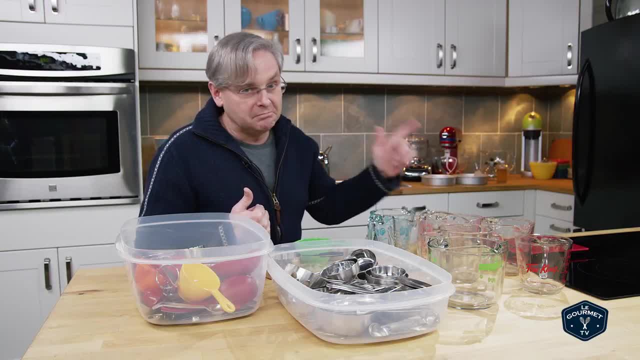 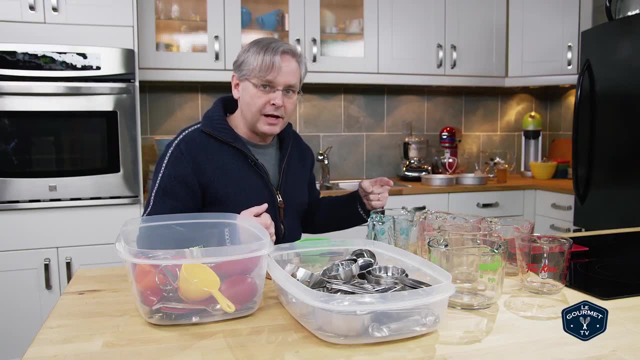 and wet ingredients for it to work. Second choice should be to find recipes that weigh the dry ingredients. That's always my first choice. Second choice should be to use recipes that give you a metric value and just use the metric value. Very repeatable.